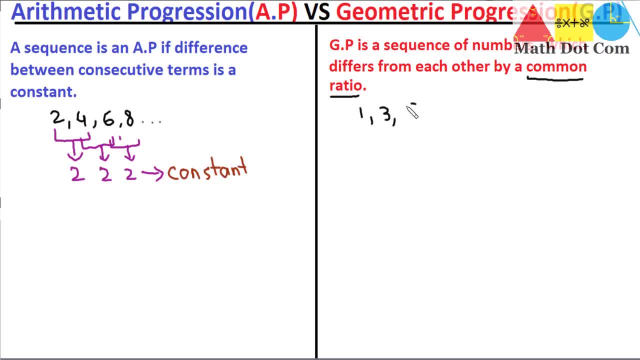 So if I write a sequence that is 1,, 3,, 9,, 27,, 51 and so on and so on, This is a geometric progression or geometric sequence. Why it is a geometric progression? Because what we have, we have the two terms that differ from each other by a common ratio. 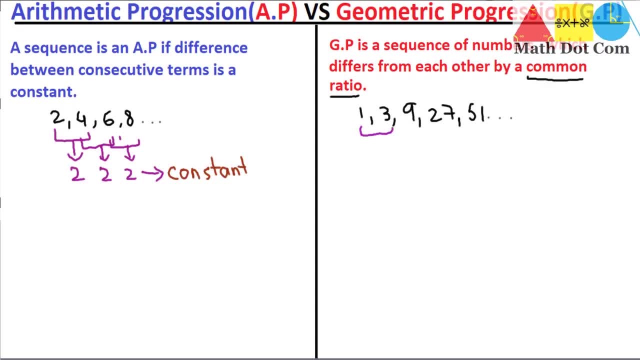 So what is meant by common ratio? For example, if we take the ratio of these two terms, what we will get is 3 divided by 1, equal to 3.. If we take the ratio of these two terms, what we will get is 27 divided by 9, equals to 3.. 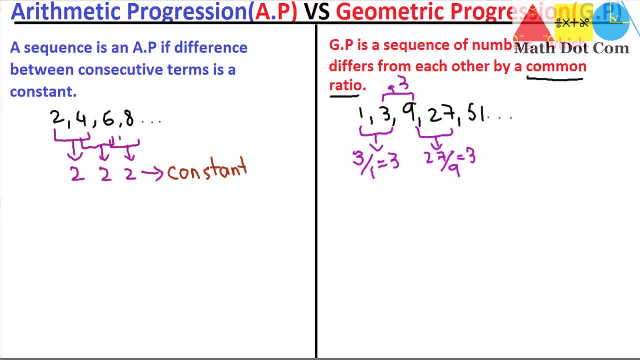 If we take the ratio of these two terms, what we will get is 3.. If we take the ratio of these two terms, what we will get is 3.. So what we have, We have a common ratio. So when you came across a common ratio, then you must say that the given sequence is a. 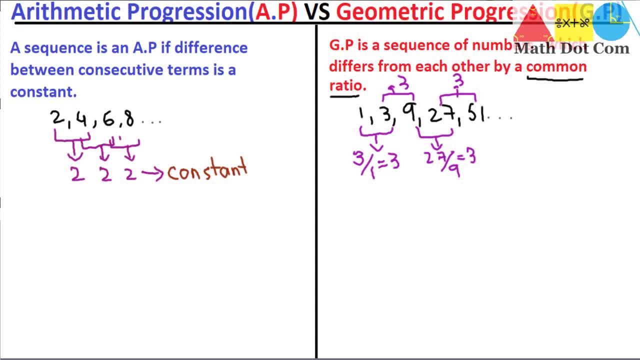 geometric sequence or geometric progression. So in arithmetic progression we were having a A common difference and here we have a common ratio. So if I write here about the common difference in common ratio, how we can find the common difference in common ratio in the 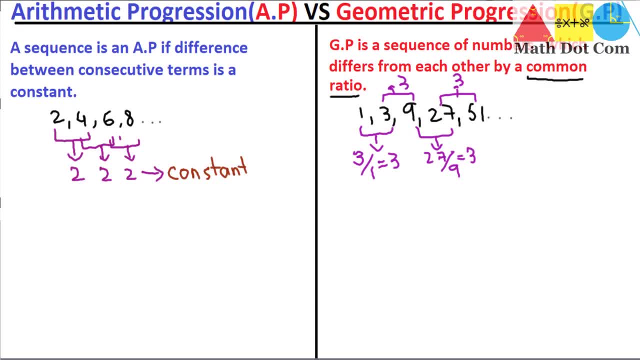 arithmetic progression and geometric progression. We also have a formula about it. Let's see So: in arithmetic progression, the common difference can be found. as so, in arithmetic progression, the common difference, or you can say a constant difference- between the two consecutive terms can be found by: as we know that the common difference is the 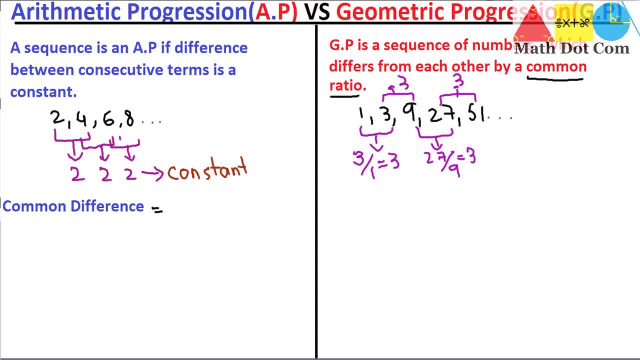 difference of the two consecutive terms in the arithmetic progression. You can say that second term minus first term and if I write better form, then you can say: the second term is a2 minus the first term is a1. and if I write in a generic way, then I can say that: 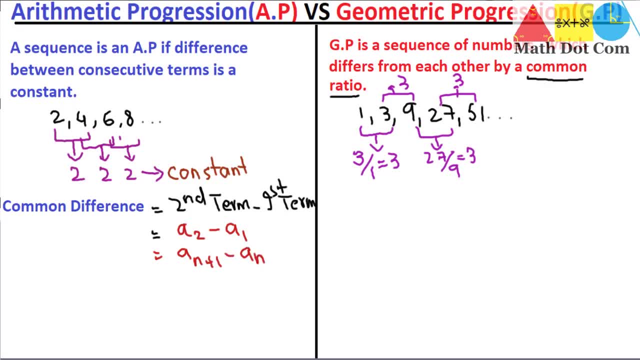 a n plus 1 minus a n. So this general formula can be used to find the common difference of any two consecutive terms. So if I write better form, then you can say that the second term minus first term is a2 minus a n. So this general formula can be used to find the 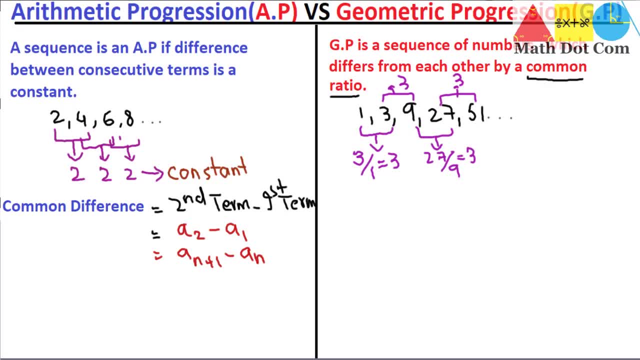 common difference of any two consecutive terms in the arithmetic progression. So this is the formula for common difference. Then if we move towards the geometric progression, then there the common ratio or the constant ratio or multiplier can be found. as common ratio or multiplier is equals to the ratio of the. you can say second term to the first. 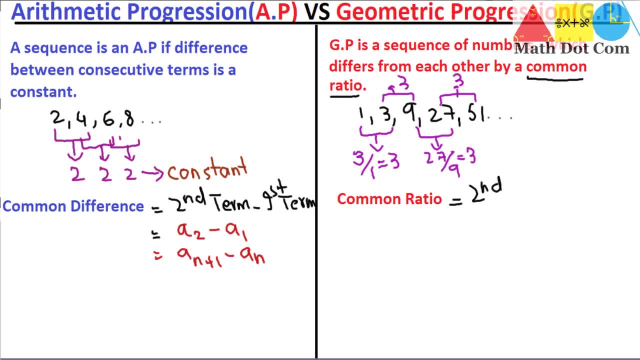 term. If I write in easy form as second term, like here, second term divided by the first term, or you can say a2 divided by a1.. Keep this in mind. you have to write the second term, first term, in the denominator and in more generic form, you can write it as a n. 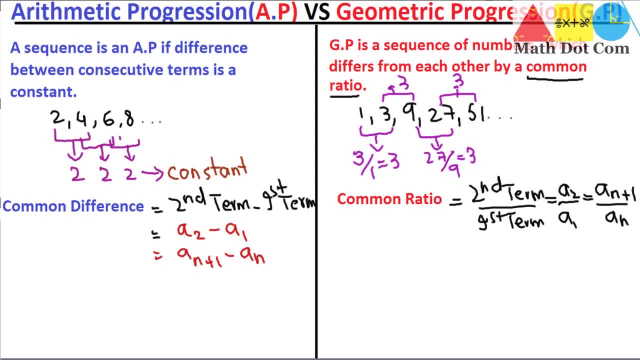 plus 1 divided by a n. So common ratio and common difference can be found by these formulas, and keep this in mind, that they are represented by D and the common ratio is represented by R. R is equals to a n plus 1 divided by a n. So this is how they differ from each other. 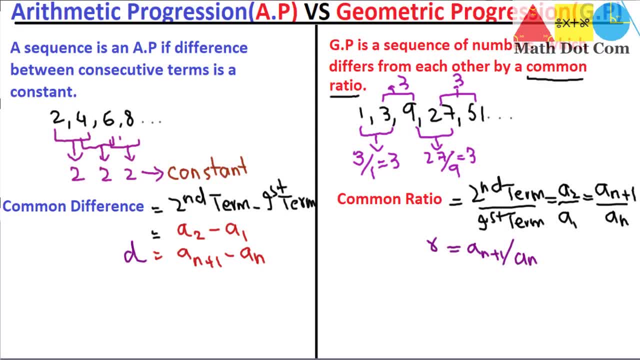 So now we must have a common ratio and common ratio, which is a 2 times a: n. When we have a common ratio and common ratio, what do we have? Well, we have the common ratio and common a. now we must have a general formula that can be used to find the arithmetic progression. 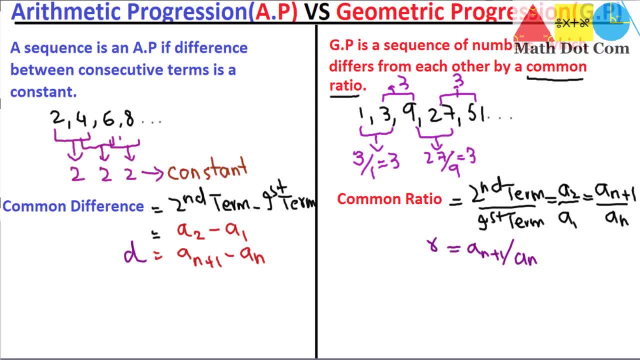 the generic form of the arithmetic progression is. that is, a general formula that can be used to find the. if you would be asked to find the second term of the arithmetic progression, or n term of the arithmetic progression, or third term or fourth term, then you must have: 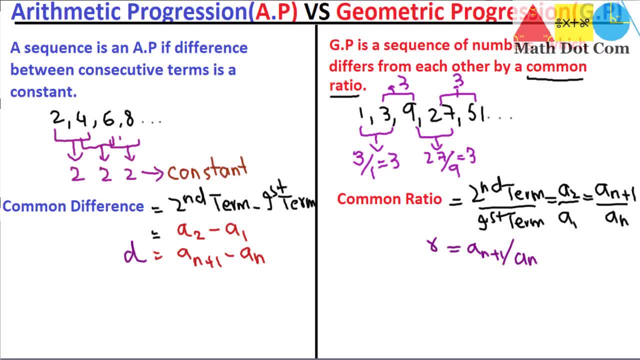 a general formula for that. So the general formula is. so general formula can be derived as if I say: if we take this example, that 2 is the first term, 4 is the second term and 6 is the third term, Now we can represent the first term by a, then the second term. 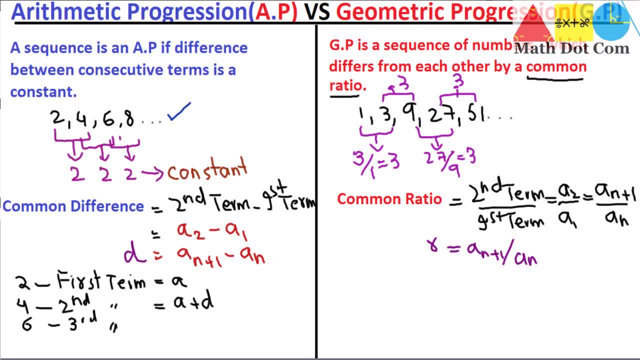 by a plus d. What is d? d is the common difference. It means when you add that common difference you will get the next term. Then the third term can be defined as a plus 2d. So it means when you move to the n number of terms you have to add the d with the multiplier It. 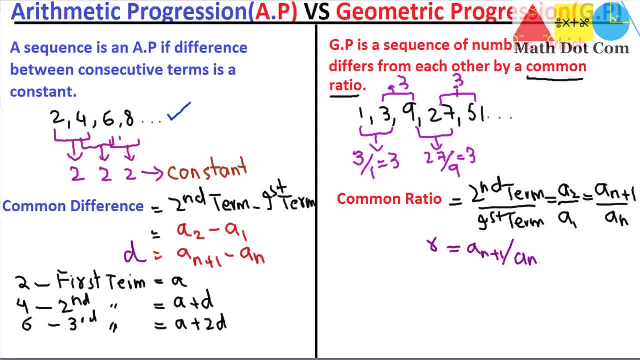 depends which term it is. So if we devise a generic form, then we can say that we can find the general form from here. as an is equals to general form, we always have the. we always have a term with n. So whenever we talk about the general term, we must represent it by 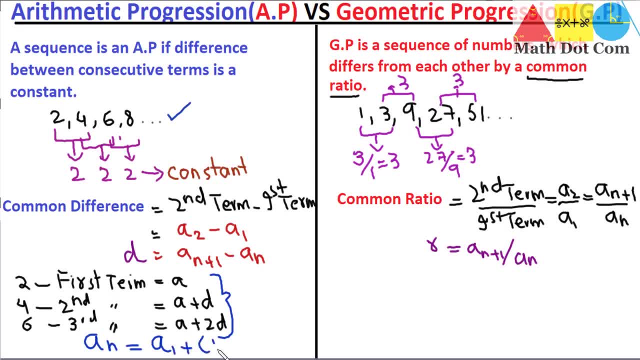 n? n is equal to a1 plus n minus 1 d. Now from where d is the common difference? and what is n minus 1?? As we move up, we are subtracting 1 from this term, So we have to divide the formula in such: 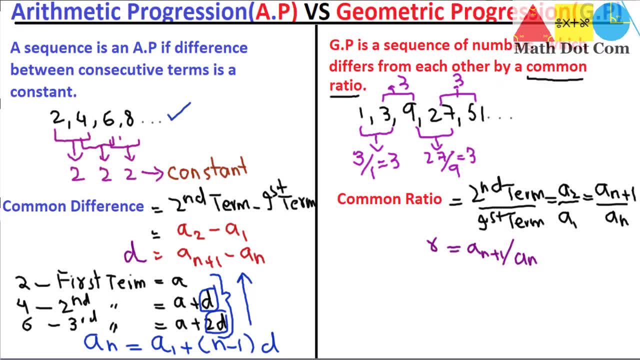 a way. So the general form of the arithmetic population is a. n is equal to a1 plus n minus 1 d, where d is the common difference, n is the number of term and a1 is the first term of the arithmetic progression. So by using this formula, you can find any term, you can find the common. 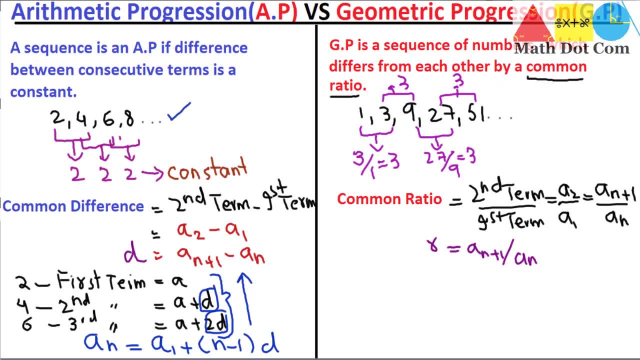 difference depends what parameters are given. Then we have the generic form of the geometric progression. For that again, we can do the same thing as from the given example. we have 1 as the first term. This is the first term of the geometric progression as given in the above example. Then 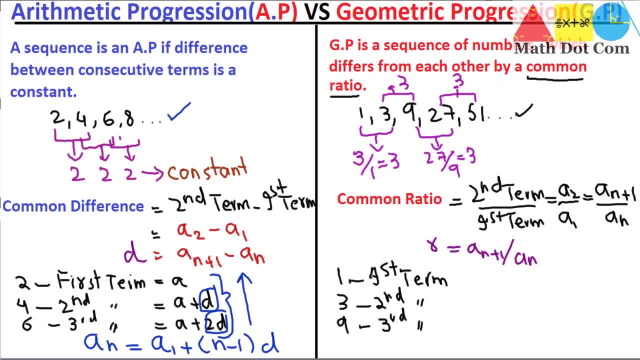 3 is the second and then 9 is the third, and so on. So the first term can be presented as a1 and the next is a12.. R, as r is the common ratio, or you can say a multiplier, It means when we multiply the given term. 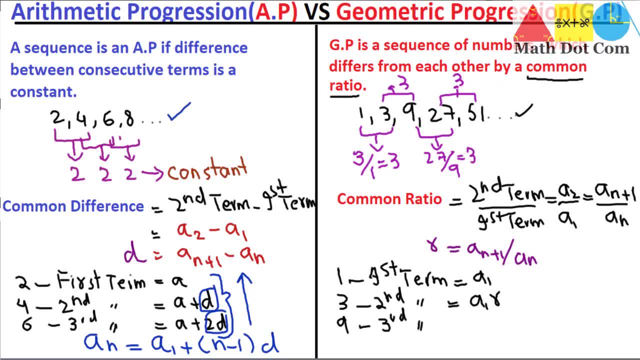 with the ratio, with the common ratio, we will get the desired term in the dramatic progression. It means we have to multiply r with the every term to get the next one. So what we will get here is a1, r2 and so on. So what will be the generic form? The generic? 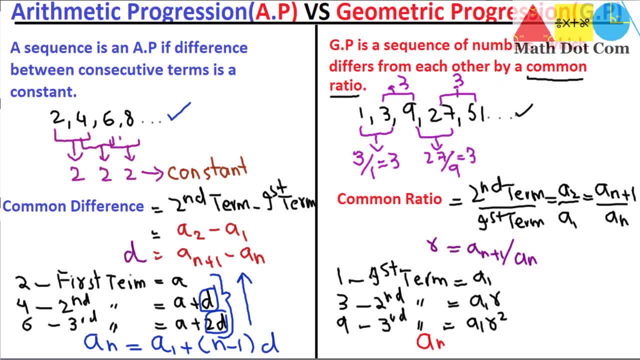 general formula of the geometric progression will be: a n is equals to a one. r raised to power, n minus one. where a n is the nth term, a one is the first term, r is the common ratio, n is the number of term, or you can say nth term if you have one, and n is equals to one. 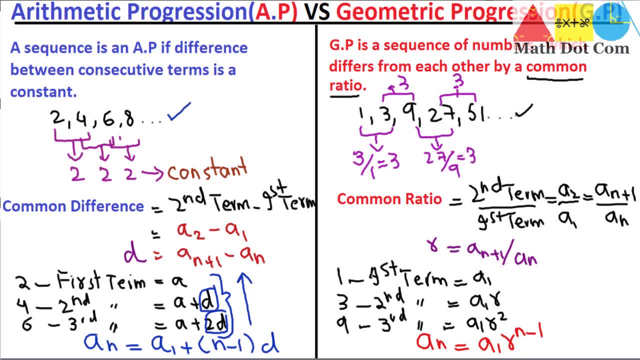 then it will be replaced by one. so how it comes out. here again, as we move up what we are doing, we are subtracting one from the power of r, though similarly we we have done the same in the general formula, as we are subtracting one from power. power of what from?